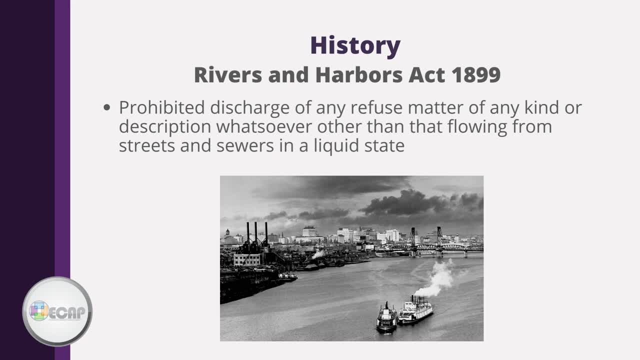 of refuse matter of any kind or description whatsoever other than that flowing from the streets and sewers, in a liquid state, into navigable waters of the United States. The primary motivation for the Rivers and Harbors Act had to do with harbors becoming difficult to navigate due to debris and trash collecting in them. 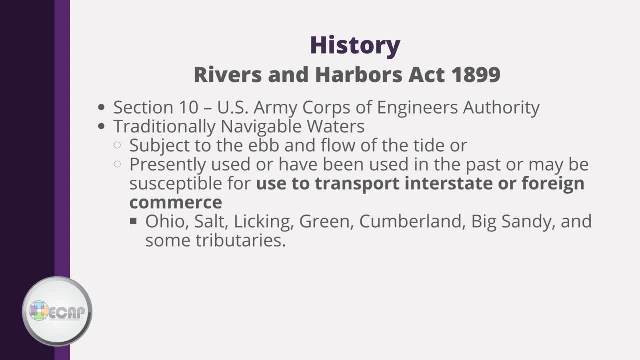 Section 10 of the Rivers and Harbors Act of 1899 gave the US Corps of Engineers authority over any activity that fills or changes any navigable water within the United States. Navigable water is a water-based water. Navigable water is a water-based water. 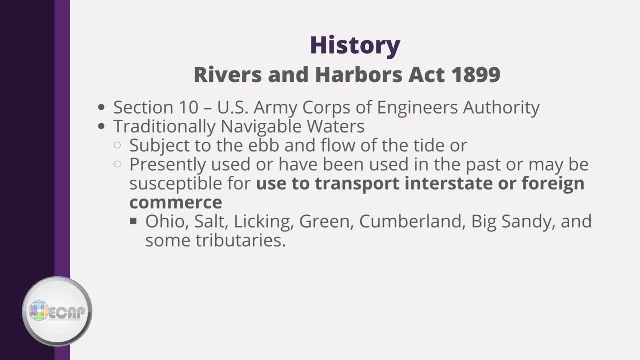 Navigable waters are those which are subject to the ebb and flow of the tide and or are presently being used, or have been used in the past or may be susceptible for use to transport, interstate or foreign commerce. Examples of Kentucky navigable waterways as recognized by the Corps of Engineers: 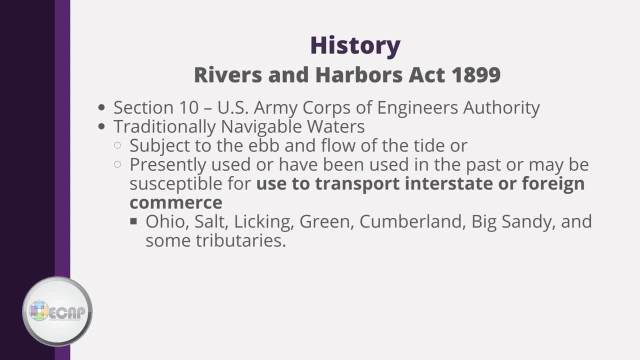 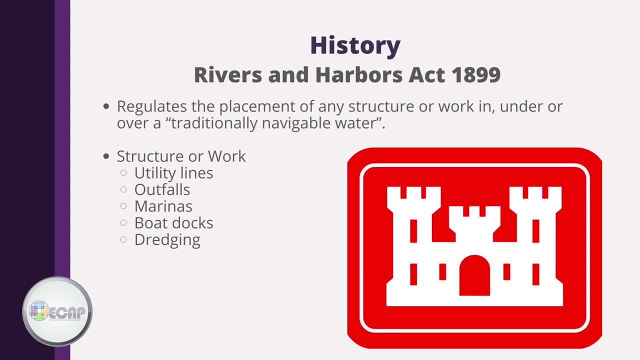 include the following rivers: Ohio, Salt, Licking Green, Cumberland, Big Sandy and some tributaries. The Rivers and Harbors Act regulates the placement of any structure or work in under or over a traditionally navigable water by giving the Corps of Engineers authority over construction excavation. 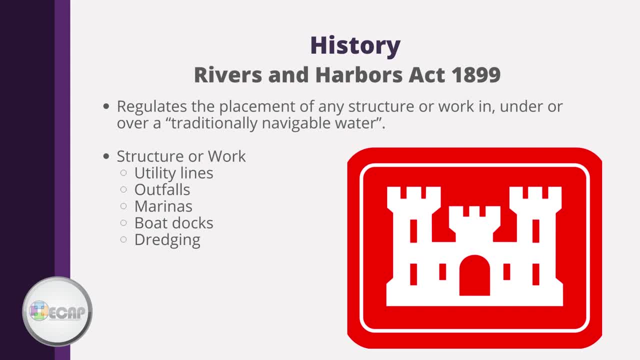 or deposition of materials into navigable waters. Some examples of a structure or work would include utility lines, outfalls, marinas, boat docks, dredging waterways and waterways. Some examples of a structure or work would include utility lines, outfalls, marinas, boat docks, dredging waterways and some tributaries. 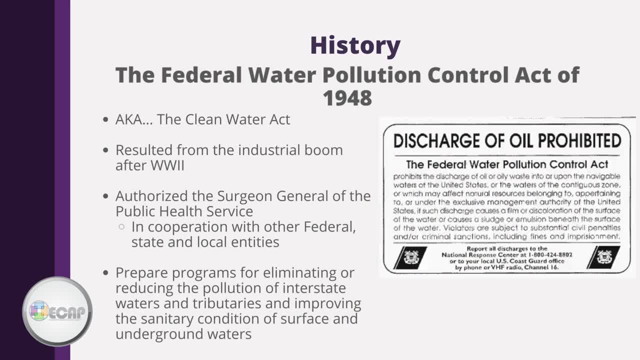 The Federal Water Pollution Control Act of 1948, or, as it is better known, the Clean Water Act, resulted from the industrial boom after World War II. Originally, this act authorized the Surgeon General of the Public Health Service, so it was a public health issue, not environmental. 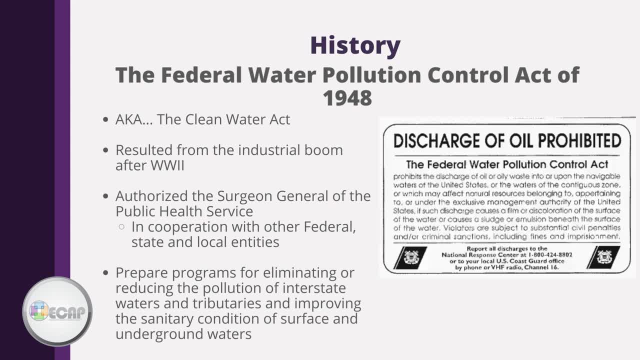 The act would require polluters to prepare comprehensive programs for eliminating or reducing the pollution of interstate waters. The act would require polluters to prepare comprehensive programs for eliminating or reducing the pollution of interstate waters in tributaries and improving the sanitary condition of surface and underground waters. 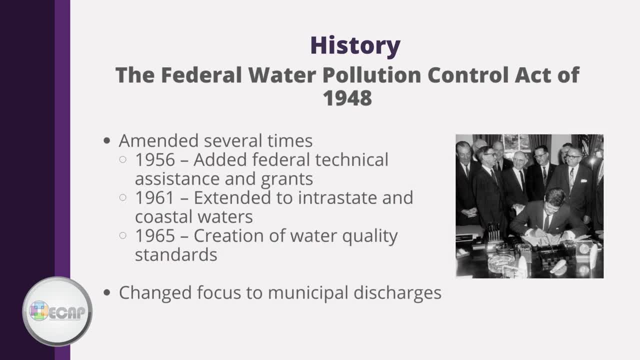 The Federal Water Pollution Control Act of 1948 has been amended several times since its inception. In 1956, amendments to the act added federal technical assistance and grants. In 1961, amendments extended coverage of the act to include intrastate and coastal waters. 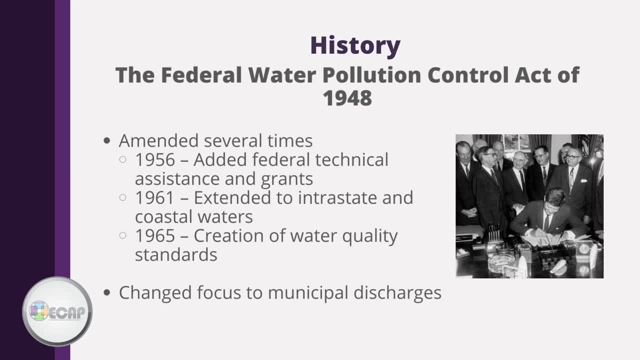 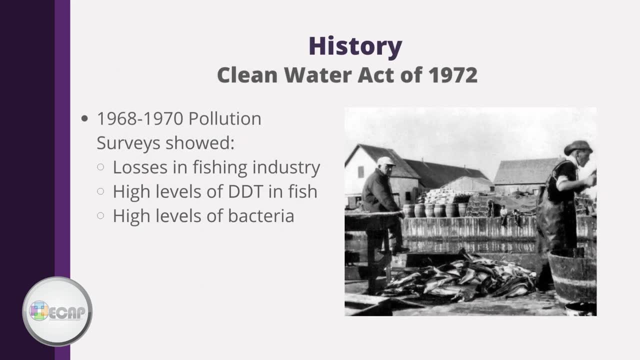 directed states to develop water quality standards. Through these amendments, the act changed its focus to municipal discharges. Pollution surveys conducted from 1968 through 1970 showed losses in the fishing industry, high levels of DDT and fish and high levels of bacteria. This period of time really brought 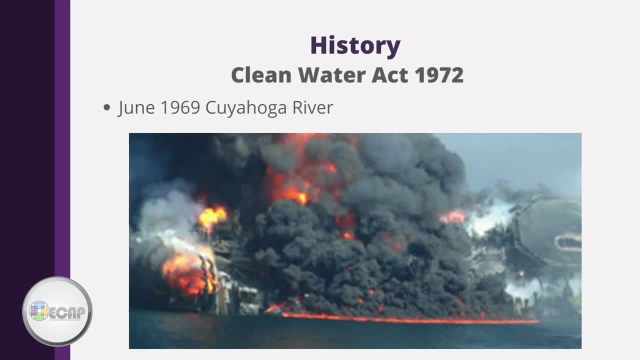 attention to the need for environmental regulations. On June 22nd 1969, the Cuyahoga River caught fire, One of the most well-known environmental disasters in US history. it spurred a lot of the environmental movement and regulations. 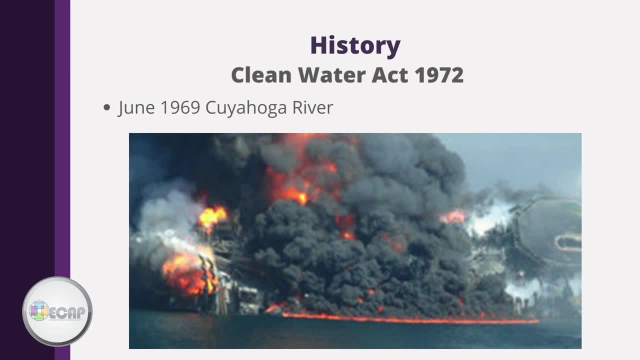 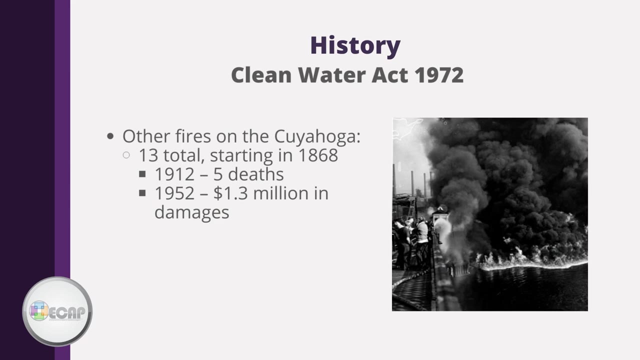 of the early 1970s, Flammable petroleum products were being dumped directly into the river by nearby industries, and the fire burned for over two hours, with flames reportedly reaching heights of over 50 feet. There have been 13 fires on the Cuyahoga River starting in 1868. The fire 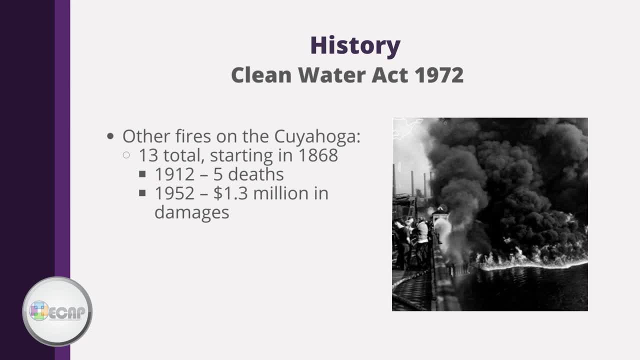 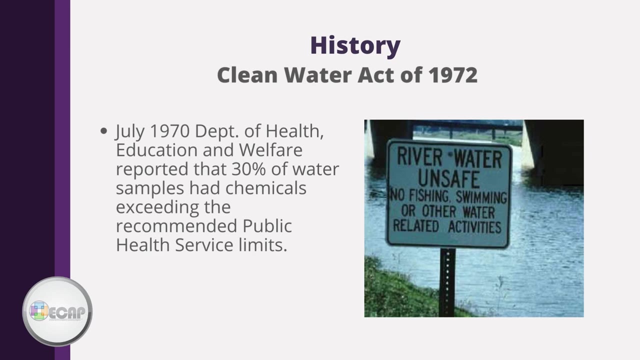 of 1912 was the most deadly, causing five deaths, while the fire of 1952 was the most destructive, causing 1.3 million dollars in damages. In July of 1970, the Department of Health, Education and Welfare reported that 30% of water 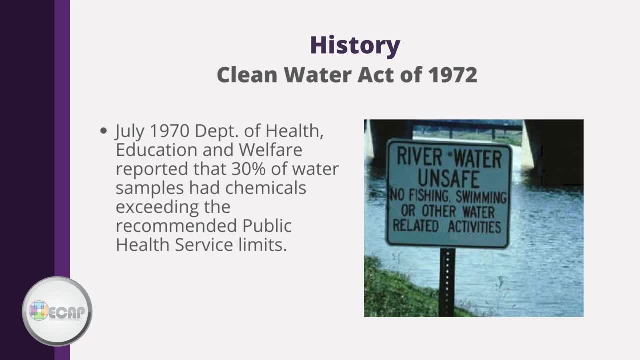 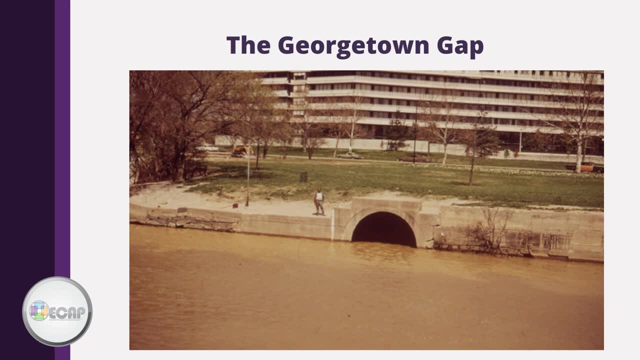 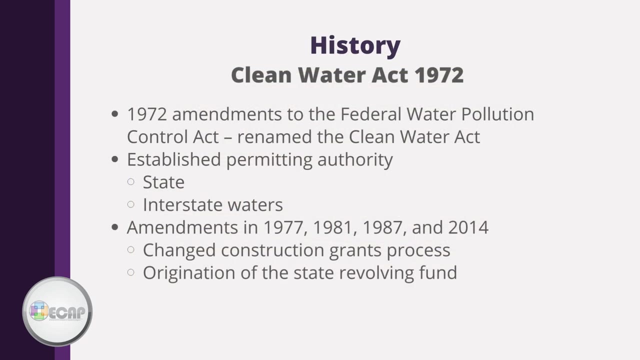 samples had chemicals exceeding the recommended public health service limits. Here we see a picture of the Georgetown Gap through which raw sewage flows into the Potomac Sites like these were common in the early 70s. The 1972 amendments to the Federal Water Pollution Control Act, which was 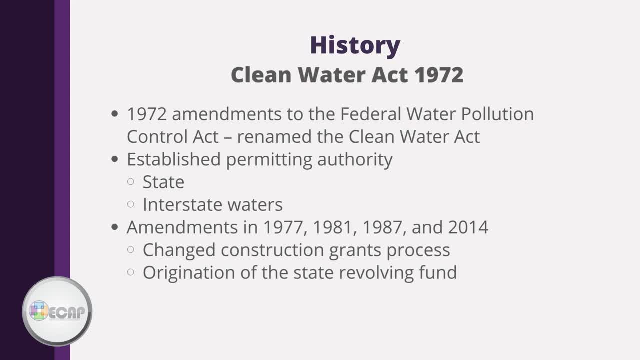 renamed the Clean Water Act, established permitting authority over state as well as interstate waters. Revisions in 1981 and 1987 were mostly about changes to the construction grant process and the origination of the state revolving fund. The Clean Water Act is broadly divided into six titles, which you can see on this. 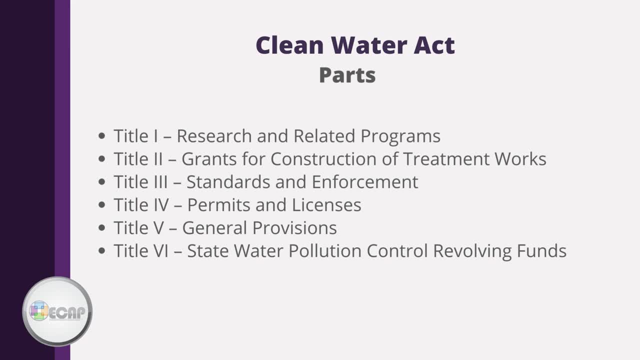 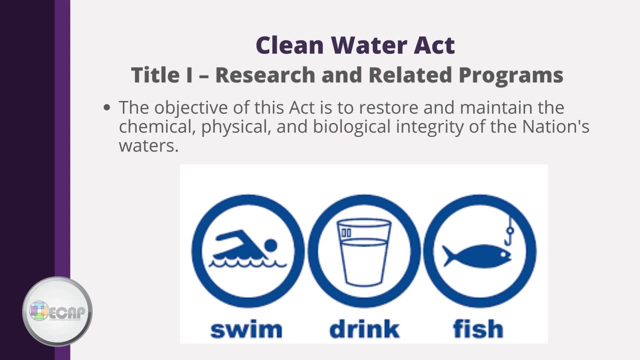 slide. We will cover each of these six titles briefly in the slides to come. The objective of the Clean Water Act is to restore and maintain the chemical, physical and biological integrity of the nation's waters. Put simply, this means the goal is to make the waters 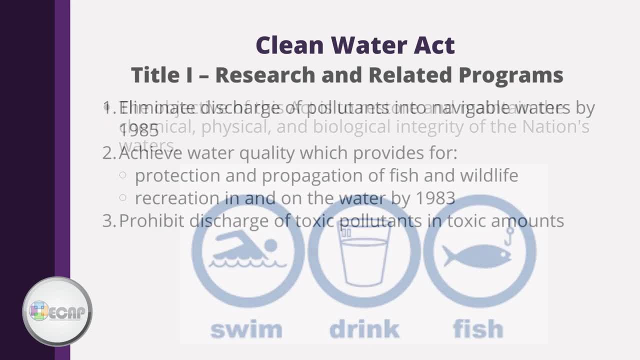 swimmable, fishable and drinkable. Title I refers to research and related programs. This title exists to provide goals for the Clean Water Act and gives guidelines on how to meet those goals. Here we can see the goals of the Clean Water Act include the elimination: 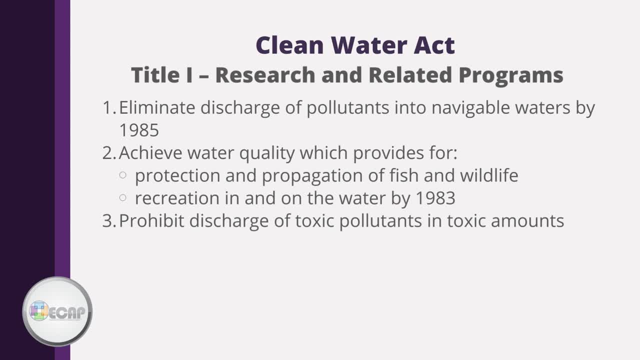 of discharge of pollutants into navigable waters by 1985.. Achieve water quality which provides for the protection and propagation of fish and wildlife and safe recreation in and on the water by 1983,. and to prohibit discharge of toxic pollutants in dangerous amounts. It is interesting to point out that they had hoped to eliminate. 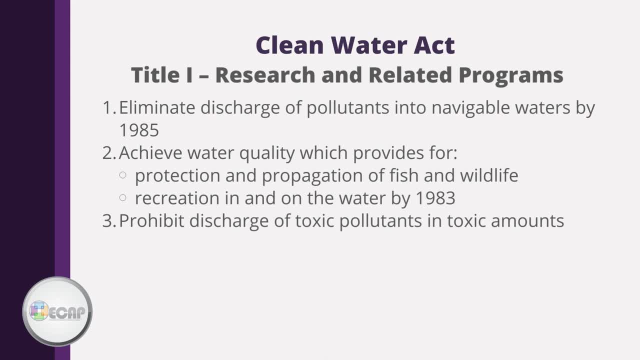 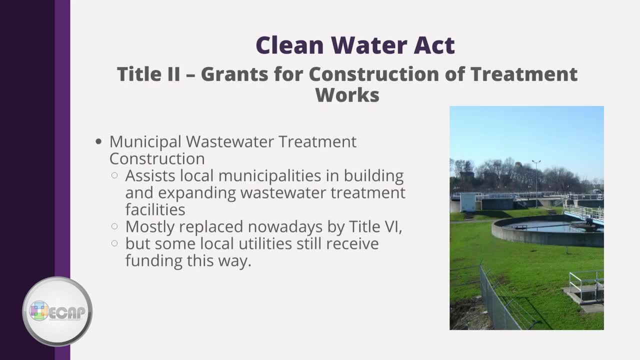 water pollution in 13 years, but we still are dealing with this issue today. Title II refers to the grants for construction of treatment works To assist local municipalities in building and expanding wastewater treatment facilities. Title II established a system of construction where federal funds would support 75% of costs. The construction grant program was replaced. 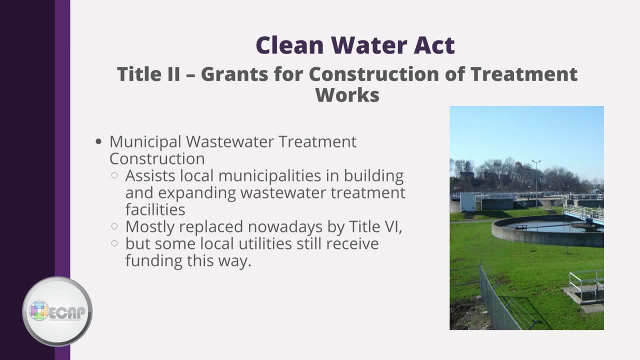 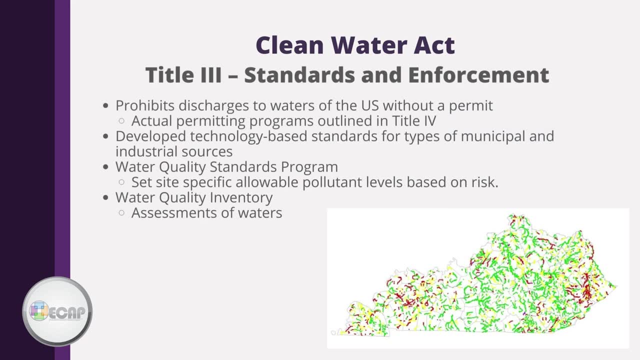 by the state revolving fund in 1987, but some local utilities still receive funding this way. Title III: Standards and Enforcement. Title III does many important things. It prohibits discharges to water of the US without a permit. Actual permitting programs are outlined. 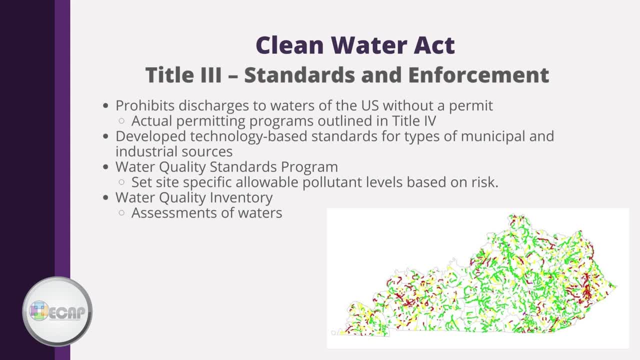 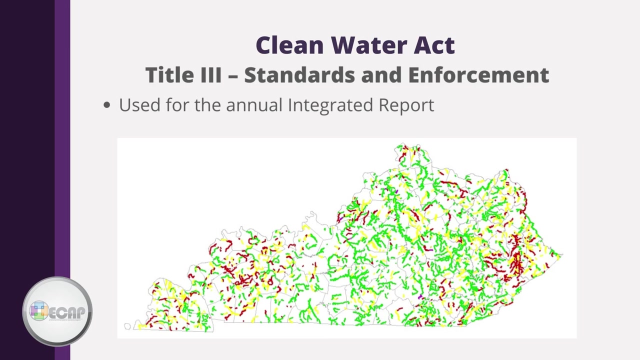 in Title IV of the Clean Water Act. It developed technology-based standards for types of municipal and industrial sources, And it developed Water Quality Standards Program, which requires states to monitor their water bodies and establish specific allowable pollutant levels based on risk. Every year, states must submit reports that describe water quality conditions to 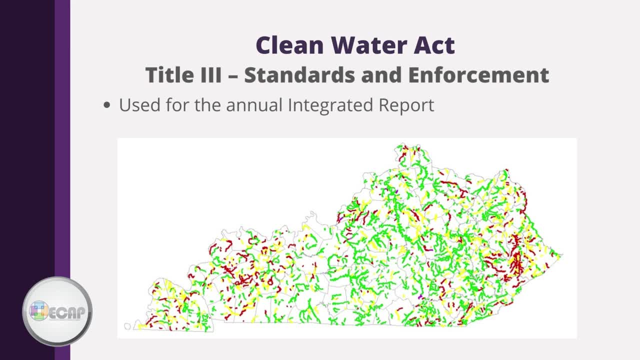 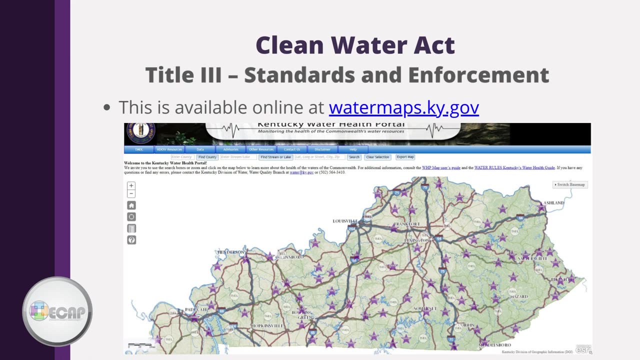 the Environmental Protection Agency. States are required to identify waters that do not, or are not expected to, meet applicable water quality standards with current pollution control technologies. The Division of Water has created an online portal where you can look up the health of any stream in Kentucky, where applicable data is available. 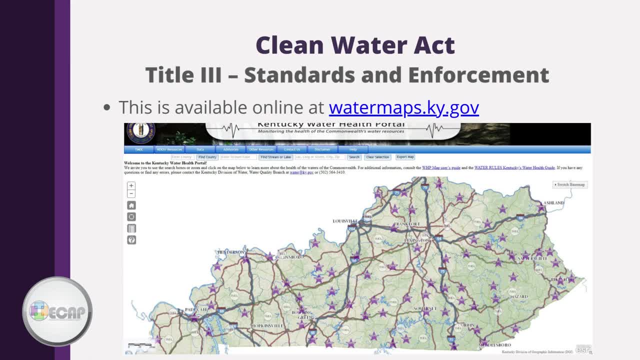 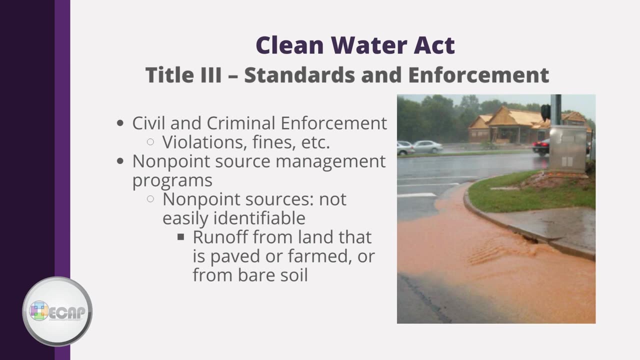 It also has a lot of other useful features, like being able to see if you are in a flood risk area or if you are in a drought. The portal is available online at watermapskygov. Title III also allows for the use of civil and criminal enforcement for water quality. 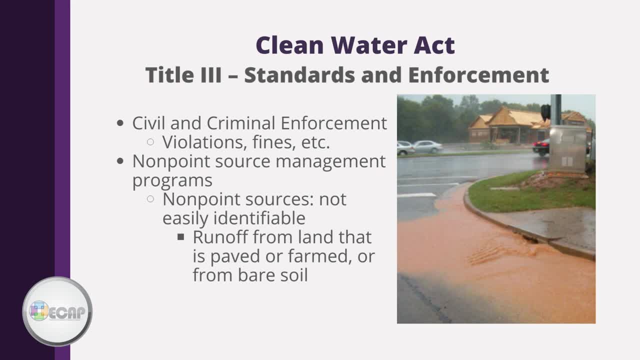 standard infractions to include violations and fines. The 1987 amendments created the Non-Point Source Managementソnate фор pp, которой создать non-point source management program overcoming surface pollution, pollutionaccessibility n, which provides grants n and supports education, as well as training n and technical assistance. 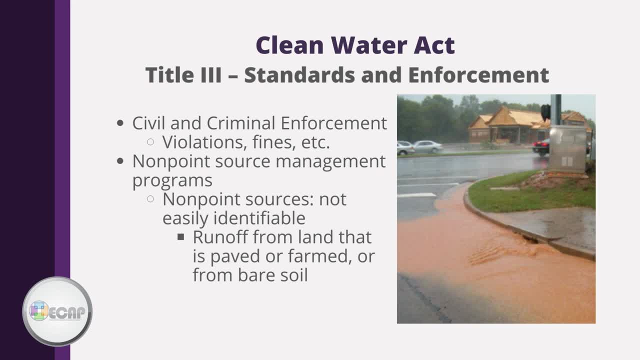 to help reduce non-point source pollution. S O s nontri sutate fn. P subquota of�kyvee. non-point sources balls nor ctinko localities na non point source pollution. Nonpoint sources are not easily identifyable and can include such things as runoff from land that is paved or farmed or from bare soil. 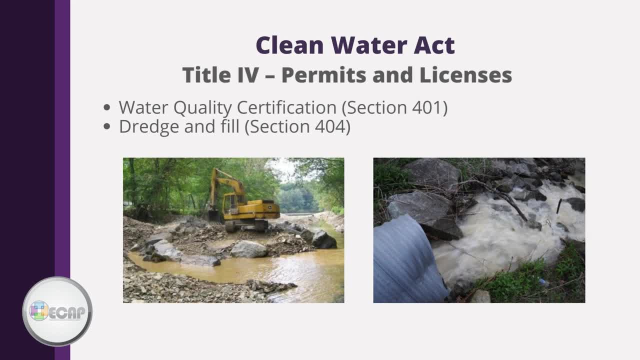 Title IV refers to permits and licenses. Section 401, the Water Quality Certification, and Section 404, Dredge and Fill are both vital parts of the Clean Water Act. Section 401 requires certification for any activity that may result in a discharge of a pollutant. 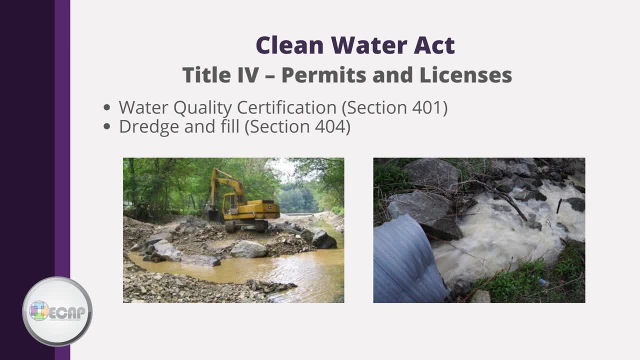 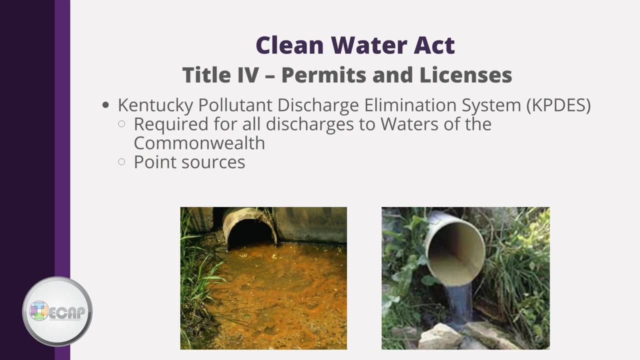 into waters of the United States And Section 404 regulates the discharge of dredged or filled materials into the waters of the United States to include wetlands, Kentucky Pollutant Discharge Elimination Systems. KPDES permits are required for all discharges to waters of the Commonwealth. 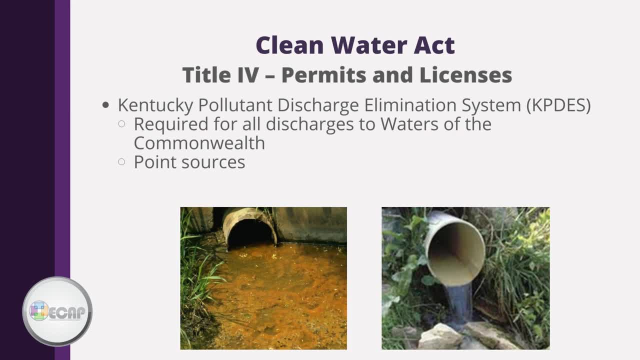 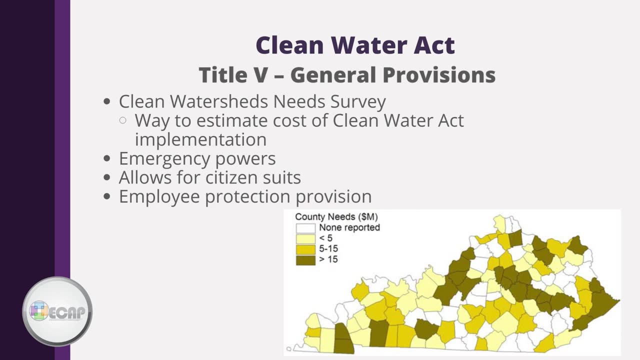 We talked about non-point sources earlier, and here we can see examples of point sources. These are discharges that come from a single point, such as a sewage treatment plant outfall or an industrial discharge. Title V of the Clean Water Act covers general provisions. 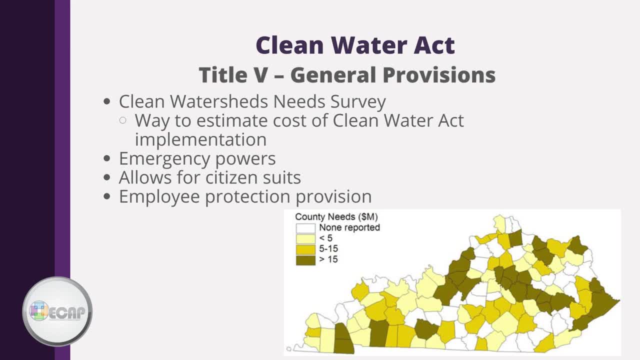 These include the Clean Watersheds Needs Survey, which is an assessment of the costs associated with meeting water quality goals, granting emergency powers for things such as beach closings, fish kills and public health concerns, and allowing any United States citizen to file a citizen suit. 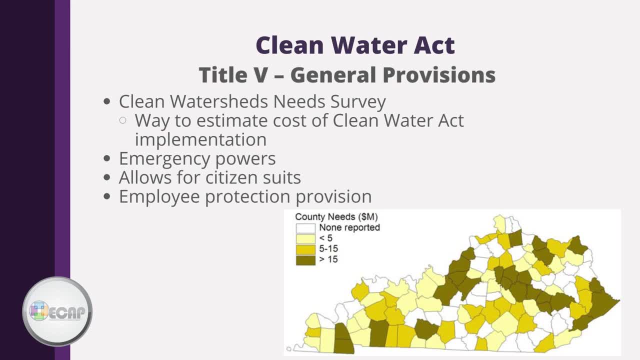 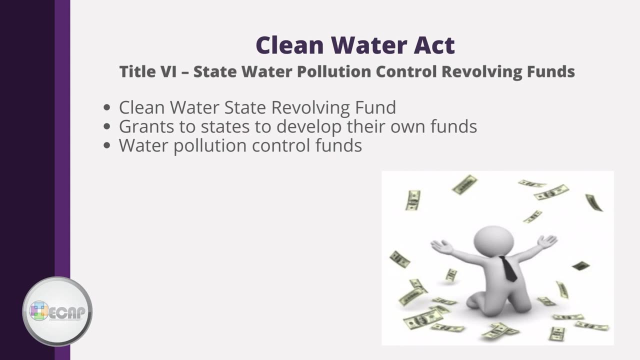 against any person who has allegedly violated an effluent limitation. Title V also contains an Employee Protection Provision. Title VI refers to the State Water Pollution Control Revolving Funds. The EPA provides grants to local states, while the state contributes an additional 20%. 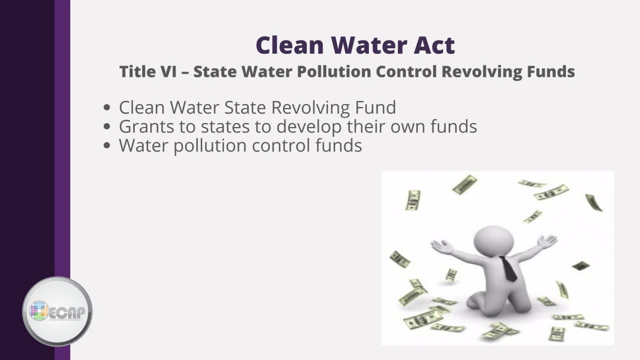 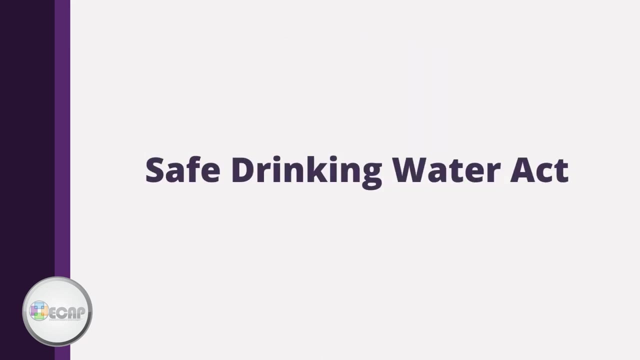 The Clean Water State Revolving Fund is a federal-state partnership that provides money to municipalities for wastewater treatment, pollution control and water protection. States are responsible for the operation of their State Revolving Fund program. Now we will spend some time talking about the Safe Drinking Water Act. 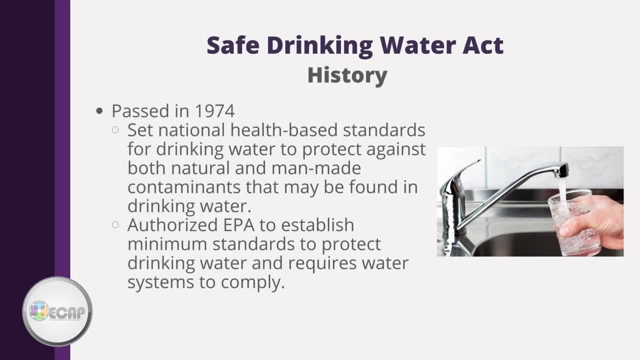 The Safe Drinking Water Act was passed in 1974, and it set national health-based standards for drinking water to protect against both natural and man-made contaminants. The law authorized the EPA to establish minimum standards to protect drinking water that water systems must comply with. 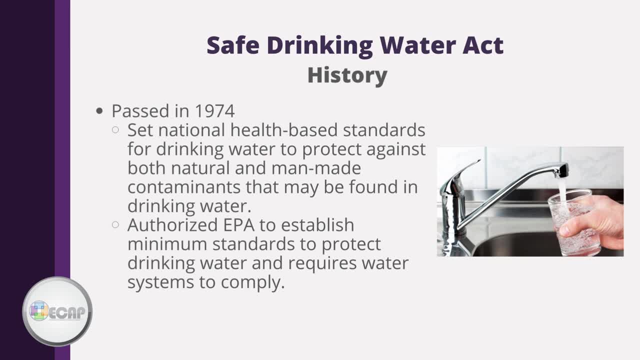 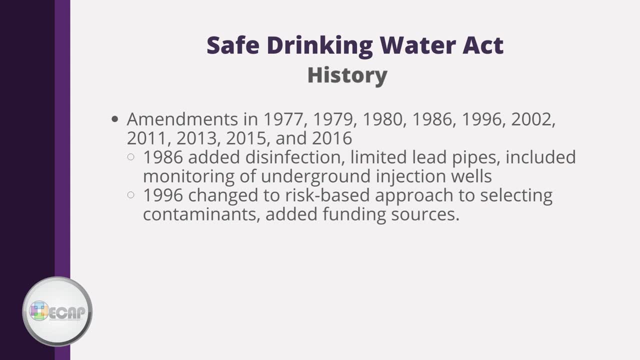 and it gave states the lead role in the implementation and enforcement of those standards. As shown by this slide, the Safe Drinking Water Act has had many amendments throughout its history. In 1986, the Act added disinfection, limited lead pipes and required monitoring of underground injection wells. 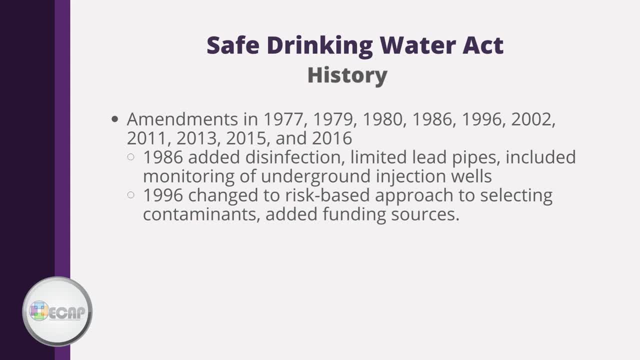 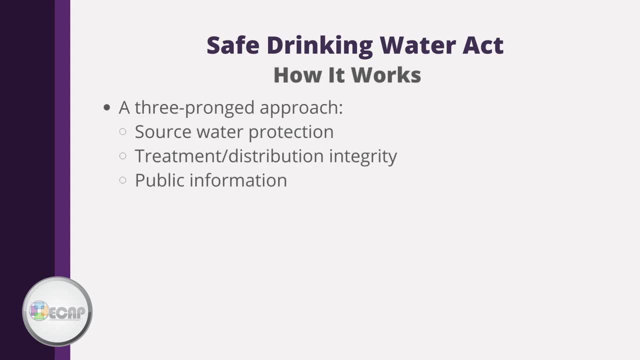 In 1996, the Act was changed to a risk-based approach for selecting contaminants and added additional funding sources. The Safe Drinking Water Act uses a three-pronged approach to ensure the water we drink is safe. First is the protection of the source water itself. 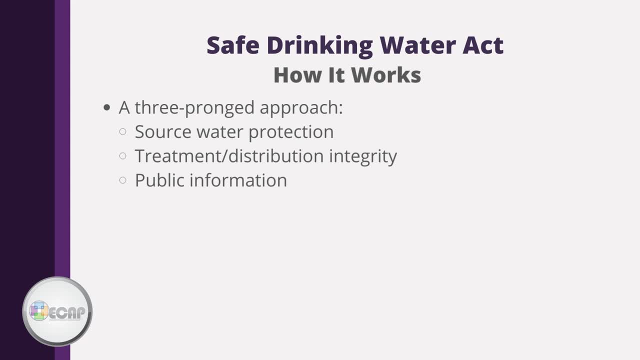 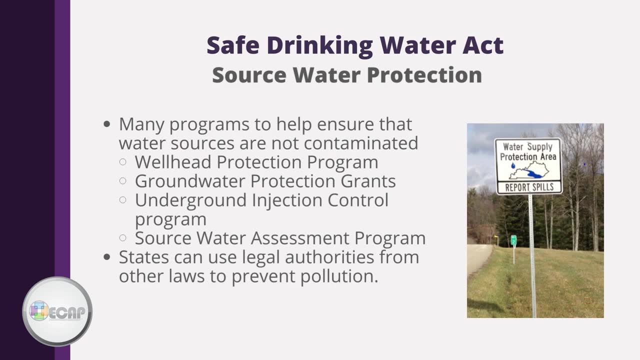 followed by measures to ensure the integrity of treatment and distribution systems and, finally, providing information to the public Source. water protection is a vital part of ensuring safe drinking water, and the Safe Drinking Water Act has several programs that help keep both surface and groundwater clean. 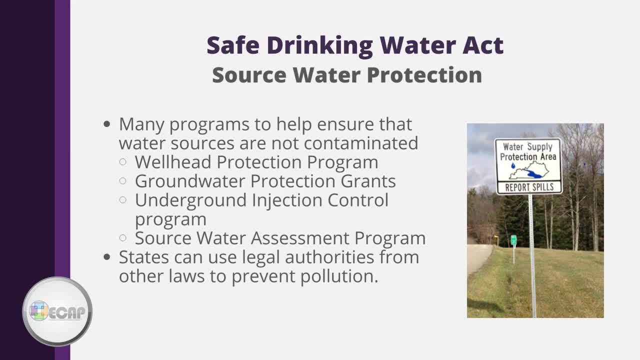 before it ever makes it to a treatment system. Wellhead Protection Program requires states to protect underground sources of drinking water. Groundwater Protection Grants, Underground Injection Control Programs responsible for Class I, IV and V injection well regulations and assuring the operation does not contaminate underground sources of drinking water. 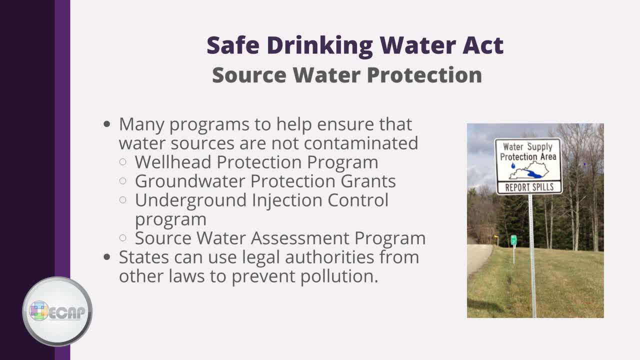 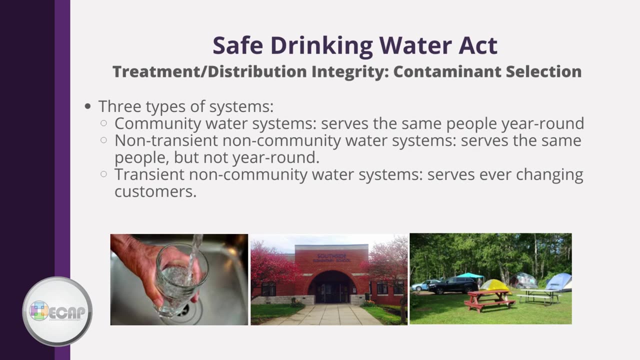 And the Source Water Assessment Program requires states to create a program for all drinking water systems to provide communities with the information required to create and enact protective measures to keep source water protected. There are three types of drinking water systems: Community water systems, which serve the same people year-round. 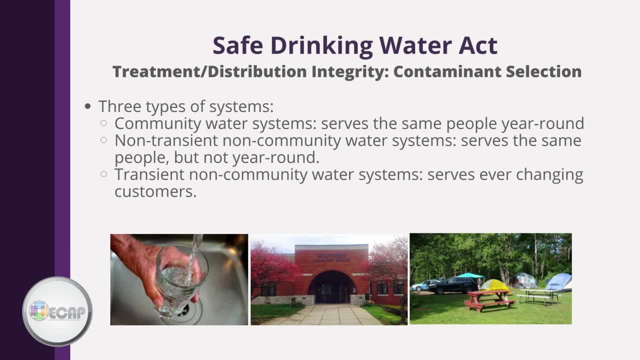 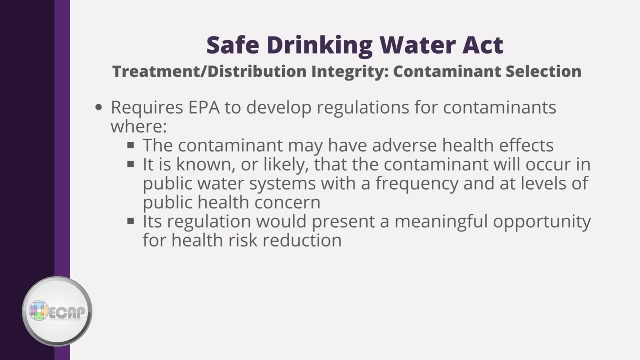 Non-transient, non-community water systems which serve the same people but not year-round, for example schools and workplaces, And transient, non-community water systems which serve ever-changing customers, such as campgrounds and gas stations. The 1996 amendments to the Safe Drinking Water Act. 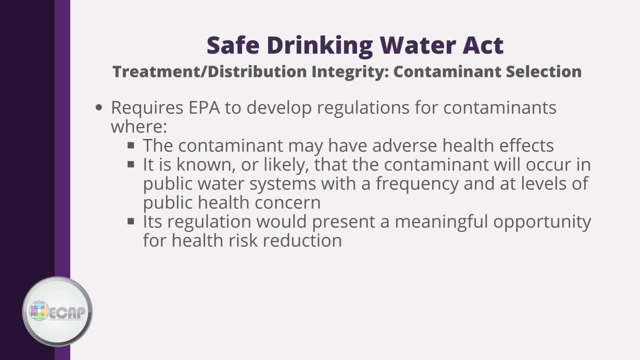 requires the Environmental Protection Agency to regulate contaminants in situations where the contaminant may have adverse health effects. In addition, the EPA must regulate contaminants where it is known or likely that the contaminant will occur in public water systems at frequency and at levels of public health concern. 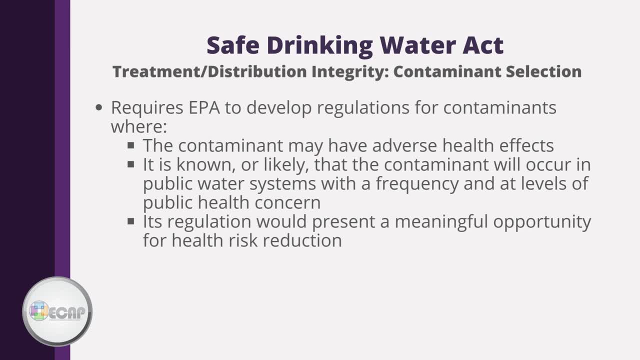 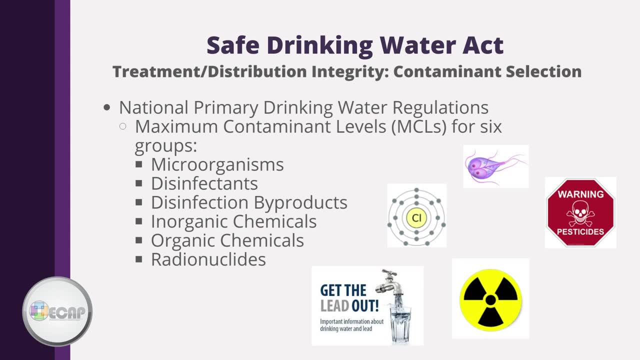 and where its regulation would present a meaningful opportunity for health risk reduction. The National Primary Drinking Water Regulations developed maximum contaminant levels for six groups: Microorganisms, disinfectants, disinfection byproducts, inorganic chemicals, organic chemicals and radionuclides. 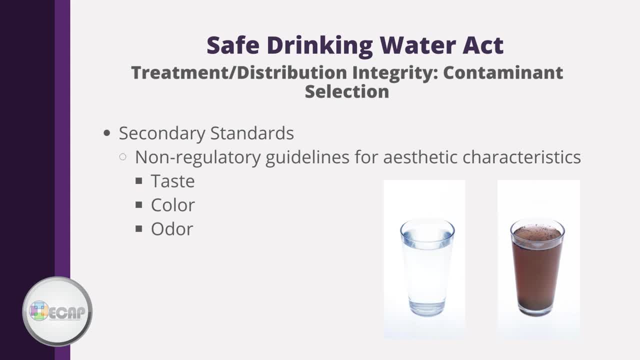 The Safe Drinking Water Act also includes secondary standards. These are non-regulatory guidelines that focus on aesthetic characteristics such as taste, color and odor. Secondary standards assume that the water still meets health-based requirements. The Safe Drinking Water Act also requires the EPA. 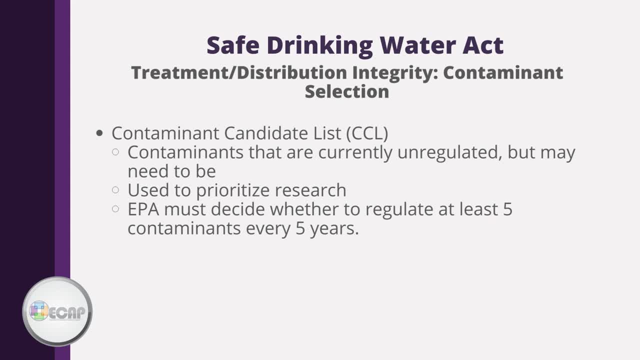 to develop a contaminant candidate list. This list consists of unregulated contaminants that may need regulation in the future and it is used to prioritize research. The list is published every five years and the EPA must consider at least five contaminants for regulation.